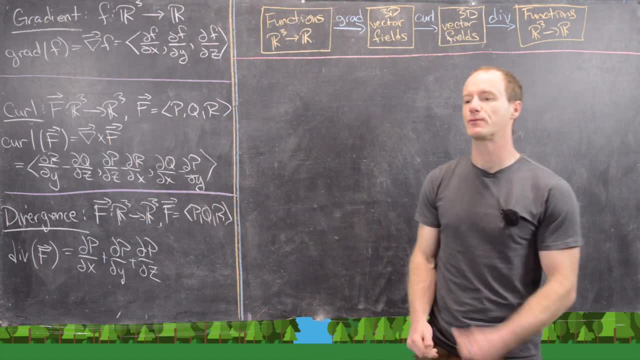 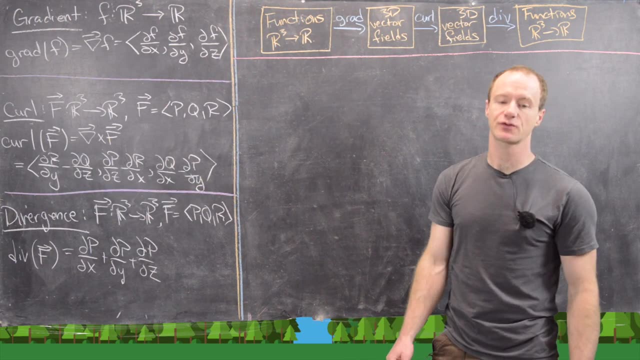 Okay, in a previous video about the vector form of Green's Theorem, we briefly looked at the notions of divergence and curl, and so we want to revisit that today, And so here we've got these three operations that can happen on multivariable functions or vector fields, as appropriate. 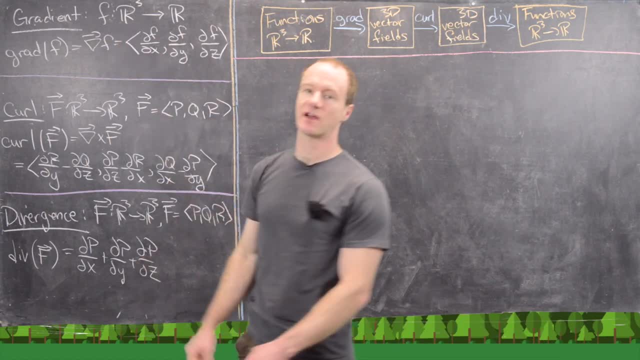 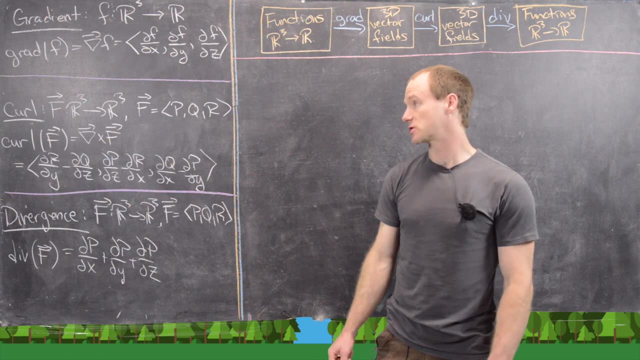 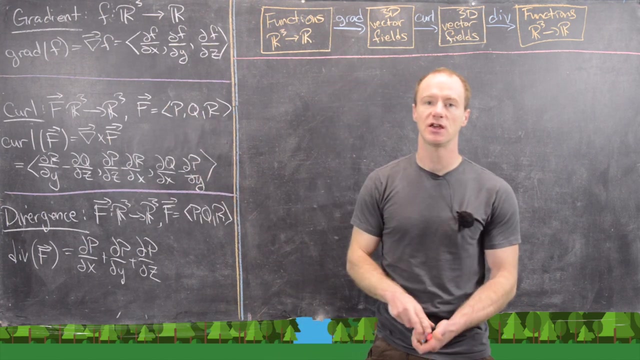 We have the gradient, and so, given a multivariable function, the gradient is a vector field made up of partial derivatives of that multivariable function. Then, given a three-dimensional vector field, so we'll call it F, with component functions P, Q and R, the curl which is sometimes denoted with just the word curl. 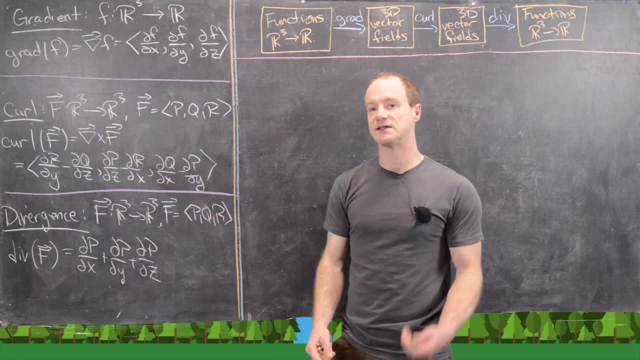 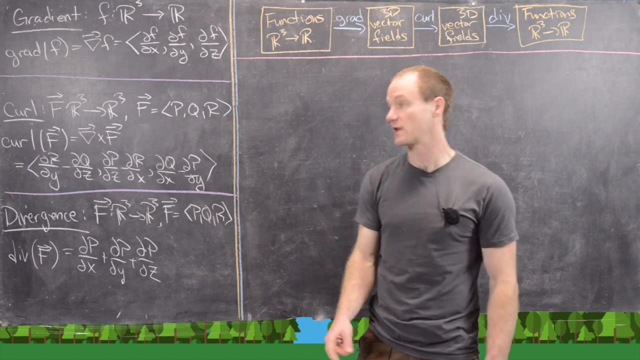 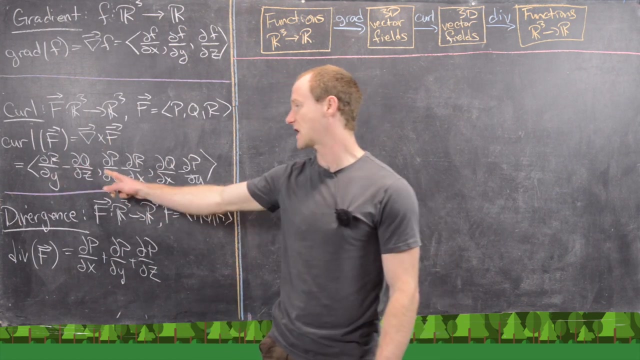 or with this del cross F, because it is almost like taking the cross product of this vector field with this differential operator which we'll see later. when we do, a calculation is given by this object right here. So we've got partial R, partial Y minus, partial Q, partial Z, comma. 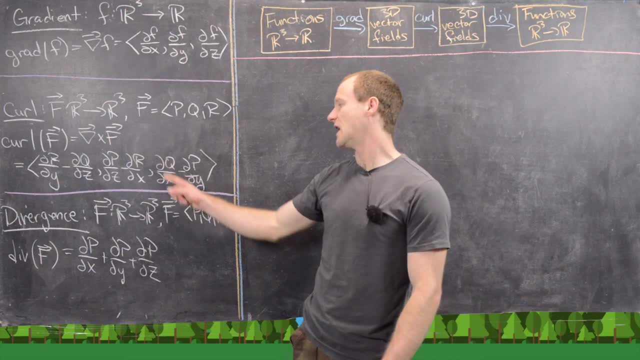 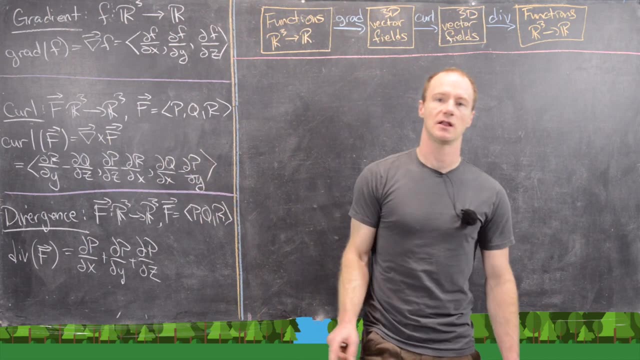 Partial P, partial Z minus partial R, partial X, And then finally partial Q, partial X minus partial P, partial Y. And notice, this part right here looks an awful lot like something that's happening within Green's Theorem. 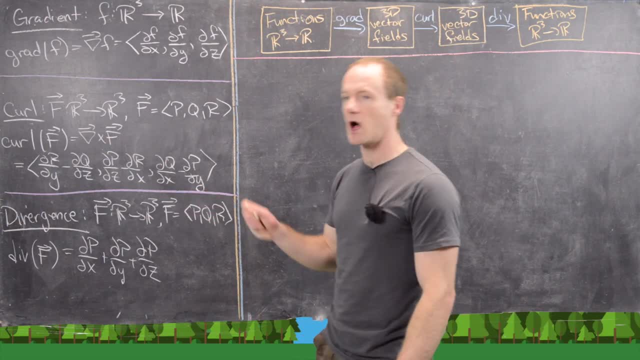 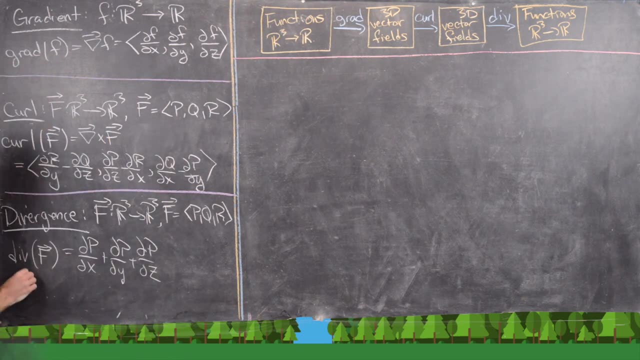 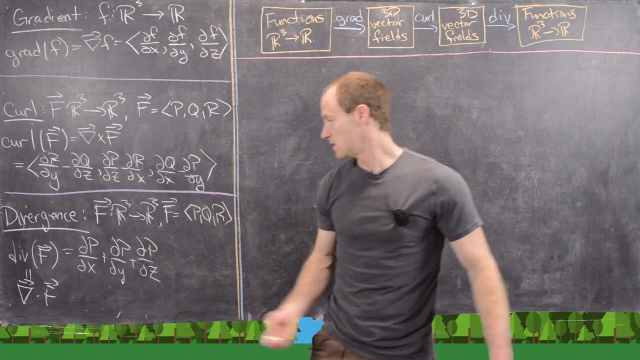 And then, finally, the divergence. it operates on a three-dimensional vector field and it gives us a function. So the divergence of F, which is sometimes written as del dot, F is partial P, partial X Plus partial Q, partial Y plus partial R, partial Z. 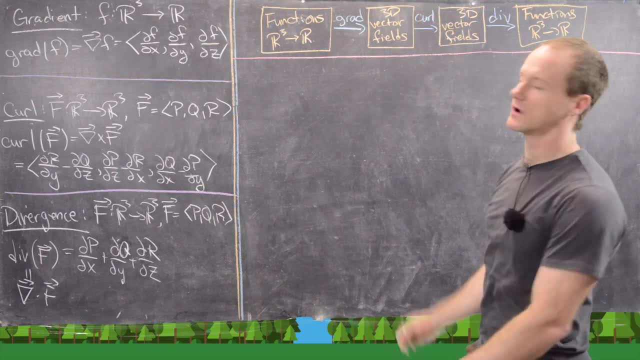 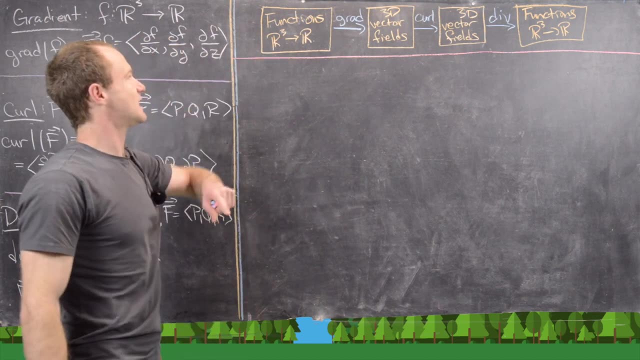 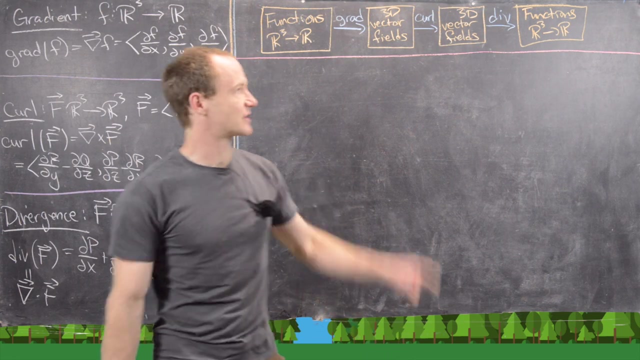 Okay, great. Now here's the picture that is really important to think about. So we have this big long string of things that's going on. So on the extreme left, we've got functions from R3 to R, Then we have three-dimensional vector fields, another set of three-dimensional vector fields and then finally, functions from R3 to R. 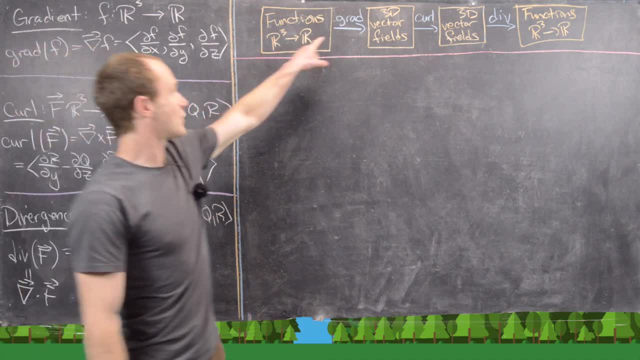 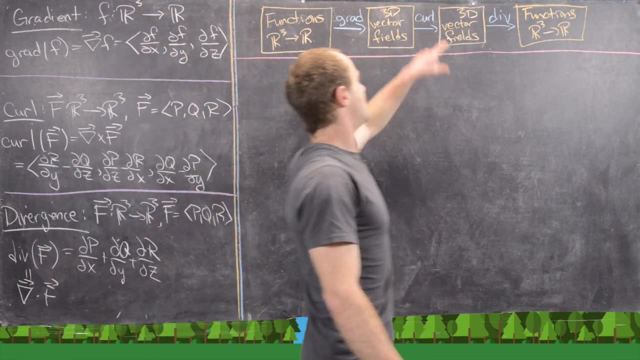 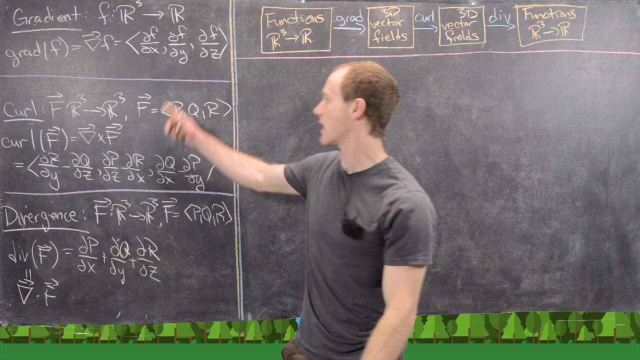 In other words functions from R3 to R. So we have functions of three variables and the gradient takes us from these functions to these three-dimensional vector fields. Then the curl allows us to stay within the realm of three-dimensional vector fields. So it goes 3D vector fields to 3D vector fields, which we can see right here. 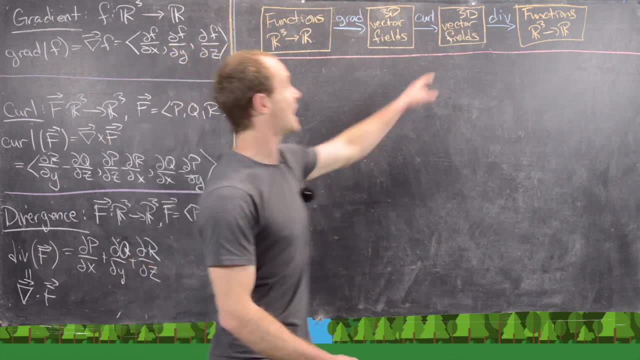 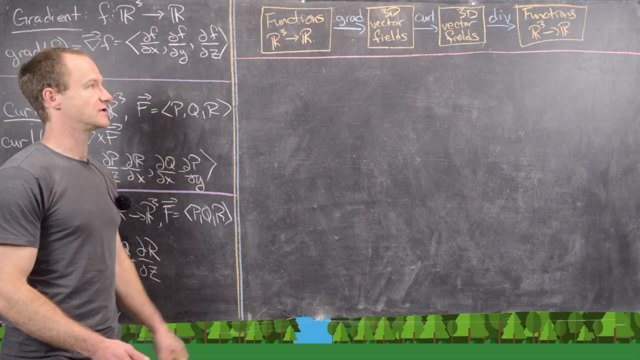 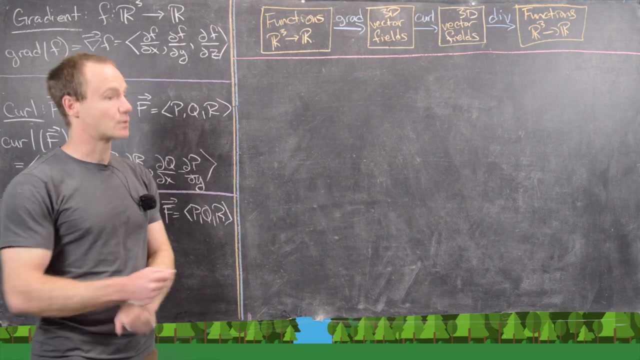 This inputs a vector field and outputs a vector field. And then, finally, the divergence takes in three-dimensional vector fields and puts out a function of three variables. And this important picture is actually happening in a larger-dimensional structure as well, which we're going to cover after we finish up the divergence there. 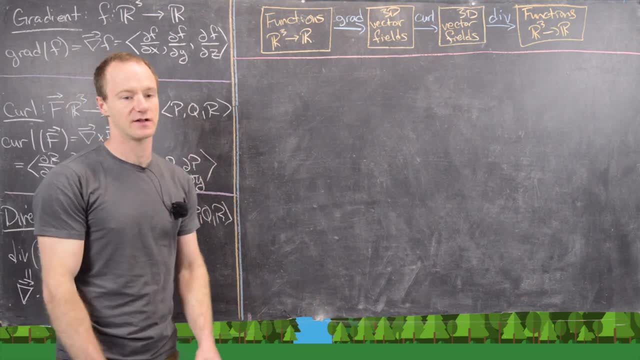 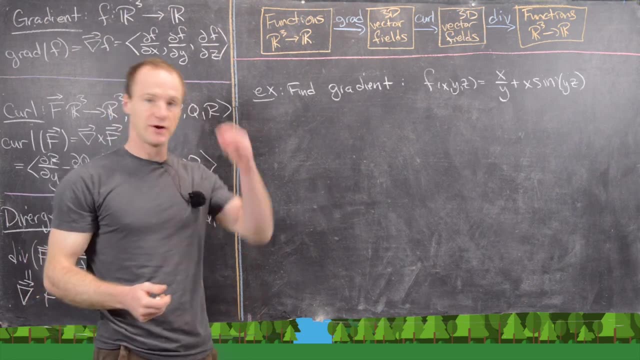 And then we're going to look at all of these notions of vector calculus in an arbitrary dimension. So stay tuned for that, Okay. so I want to do some examples real quick. Now we're going to do a quick example of each of these things. 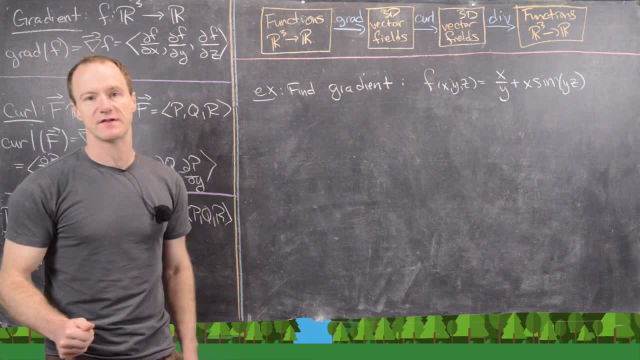 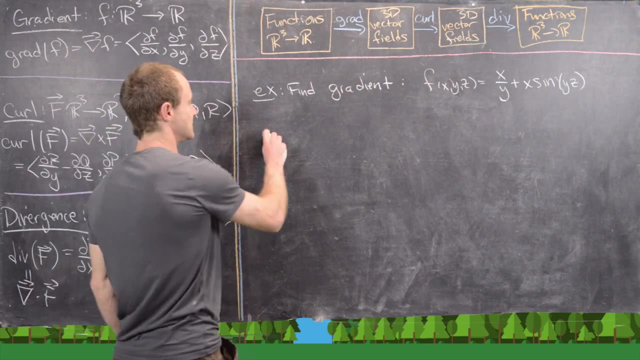 So the first one we'll do is the gradient. So let's find the gradient of this function, fxyz, which is x over y plus x, x times sin yz. So let's see Gradient of this thing. So in the first component we'll have the partial with respect to x. 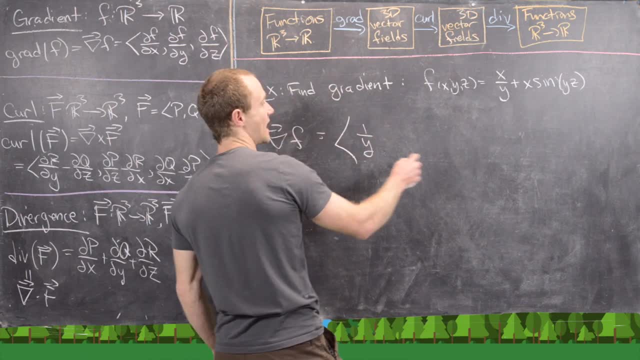 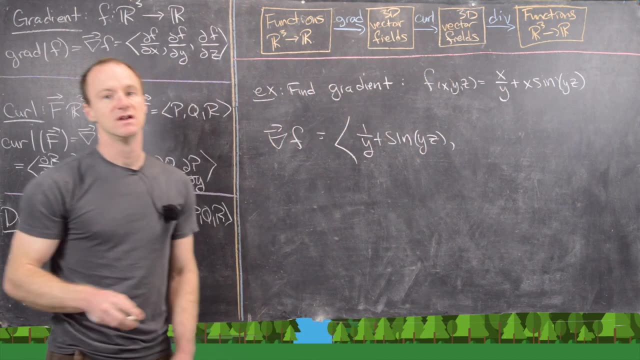 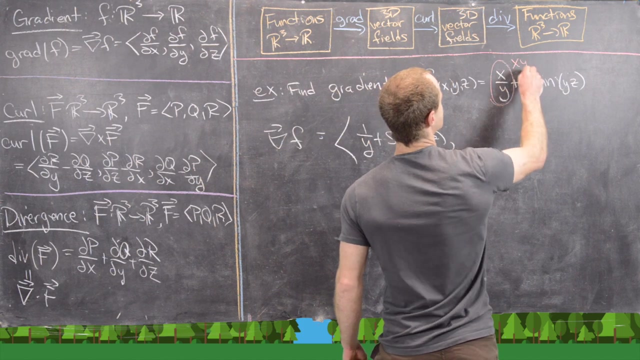 So notice, the partial of this guy with respect to x is 1 over y. The partial of the second term with respect to x is sin yz. Okay. So next we need the partial with respect to y. So now, thinking of this guy right here as x times y to the minus 1, that shouldn't be too hard to do. 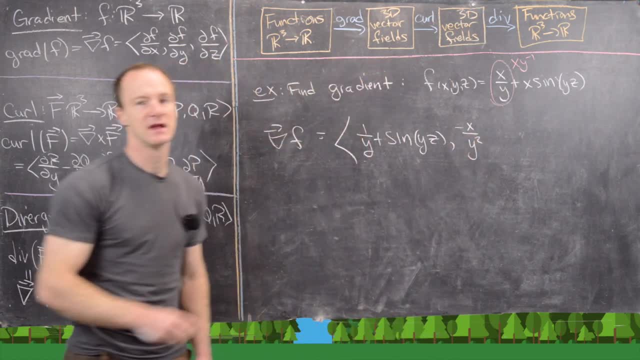 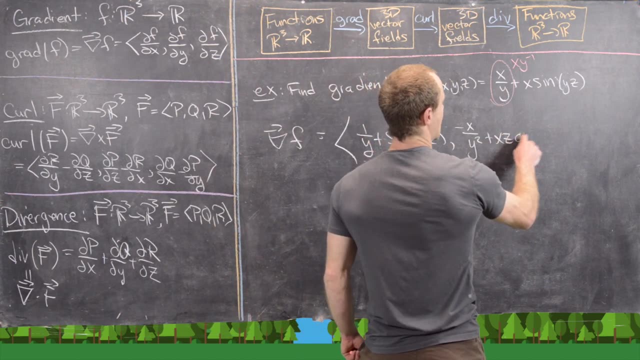 Notice that's going to give us minus x over y squared. Now we need to take the derivative of that second term with respect to y as well. That is going to be x times z and then cosine yz, where we use the chain rule as appropriate. 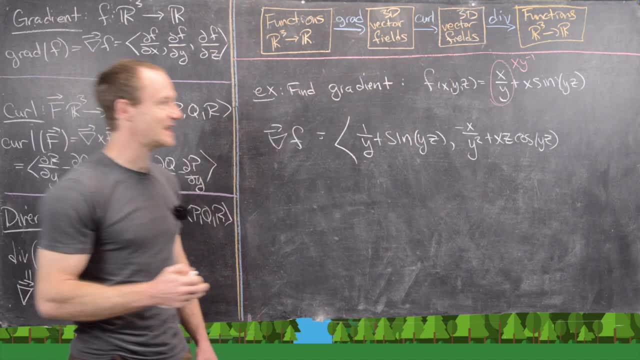 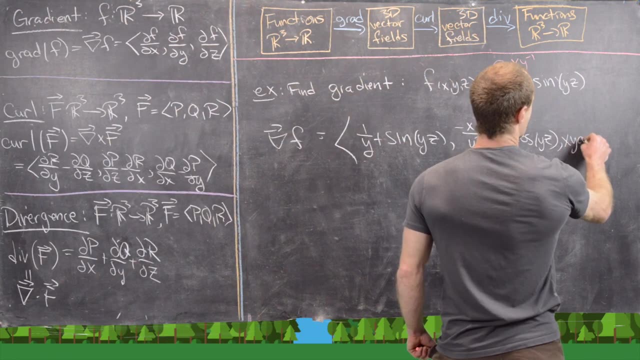 All right. Now take the derivative with respect to z. Notice, there's no z in this first term, So the derivative of that is 0.. And then we're going to get xy, cosine, yz. Okay, So that's our gradient for this function. 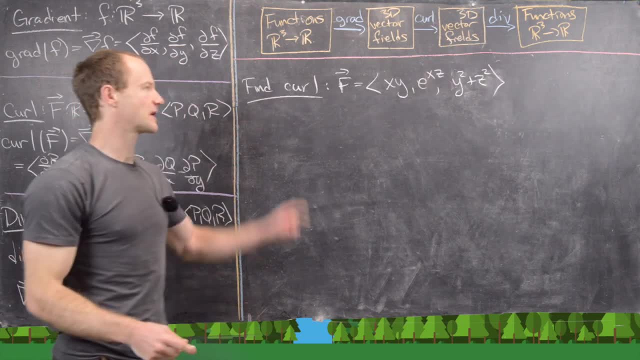 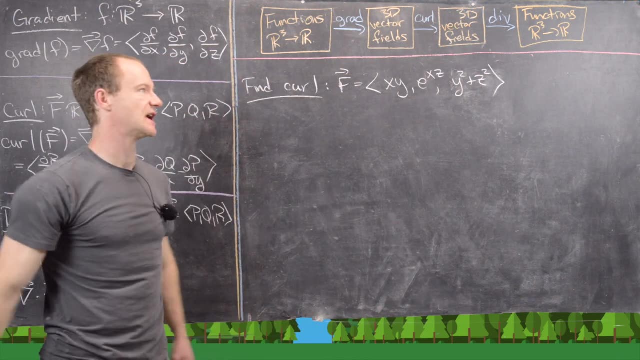 I'll clean up the board and then we'll calculate a curl. So now we're going to calculate the curl of this vector field. So its first component is x times y, The second one is e to the xz, And then the third one is y squared plus z squared. 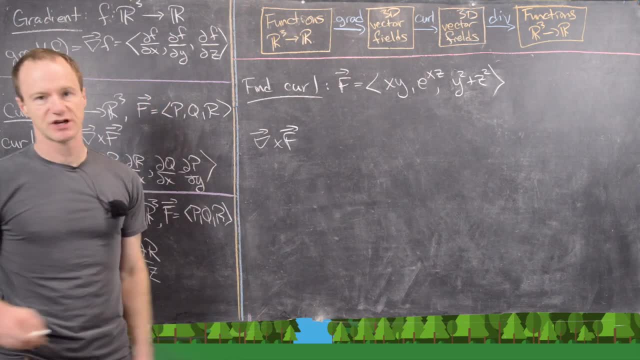 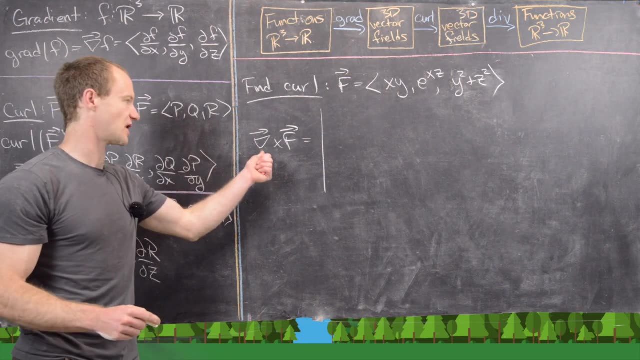 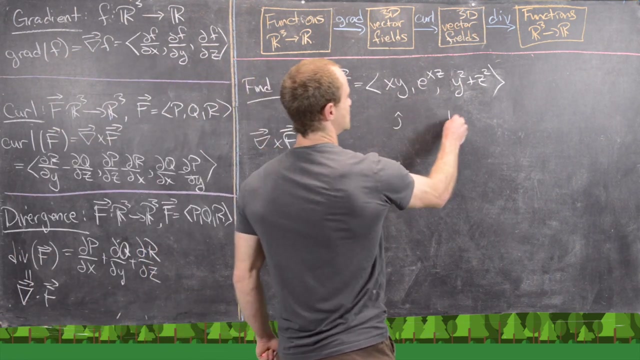 So here we'll say del cross f, We'll use that notation for the curl, And then we'll use the fact that this is nicely calculated by taking the cross product of this differential operator del with this vector field f. So in other words, we'll make this matrix i, j, k and then partial with respect to x. here 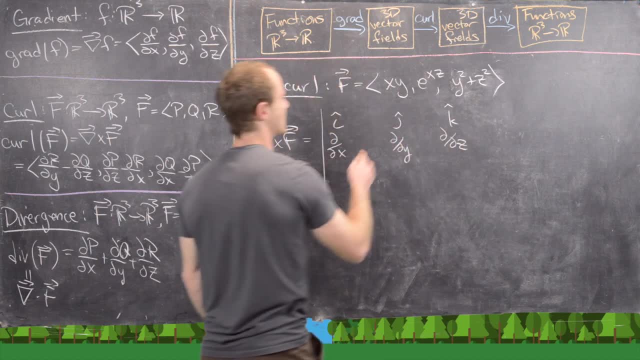 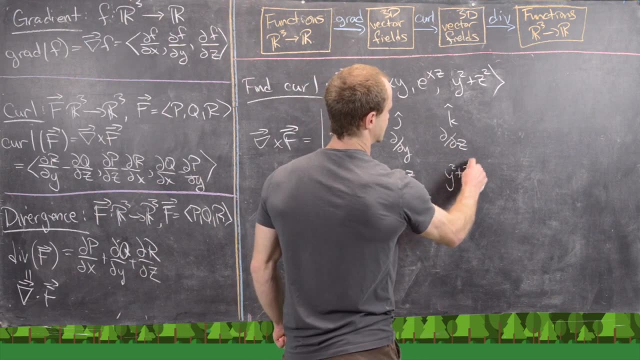 partial with respect to y here, partial with respect to z here, and then p, q and r down here. So we have xy, e to the xz, and then y squared plus z squared, And this is really loosely a matrix. 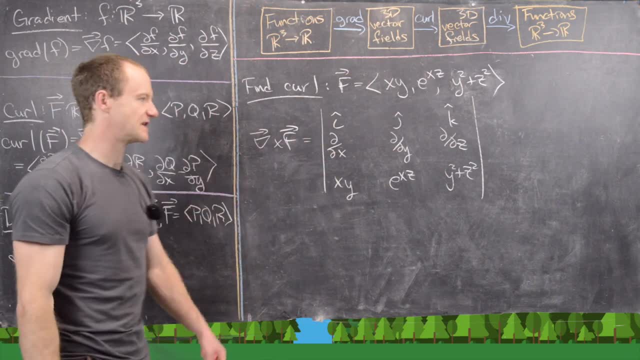 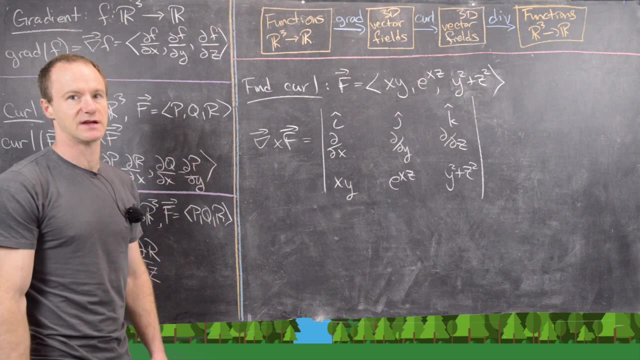 Notice, the first row is made up of unit vectors, the second row by differential operators and then the third row by functions. So this is really just a tool. So I wouldn't think too hard about this thing being a matrix or about taking the determinant. 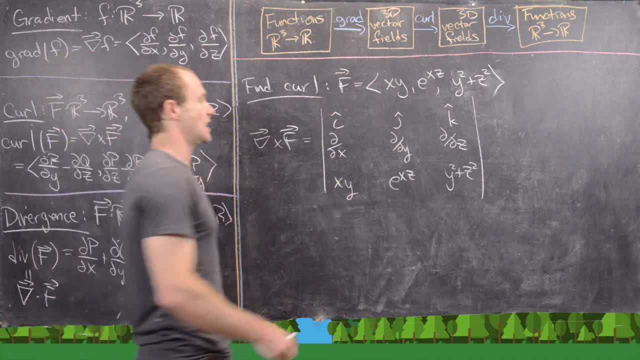 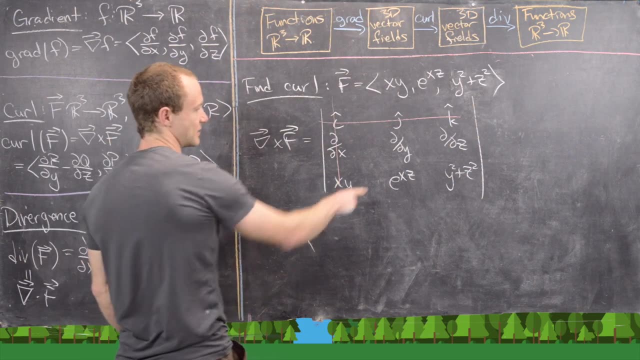 This just happens to work, Okay. so now let's go ahead and do this. So the first component we'll get by crossing the first row with the first column and then taking that determinant. So it's the partial, with respect to y, of this thing. 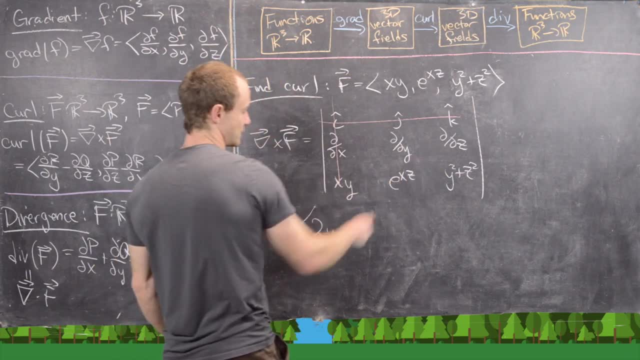 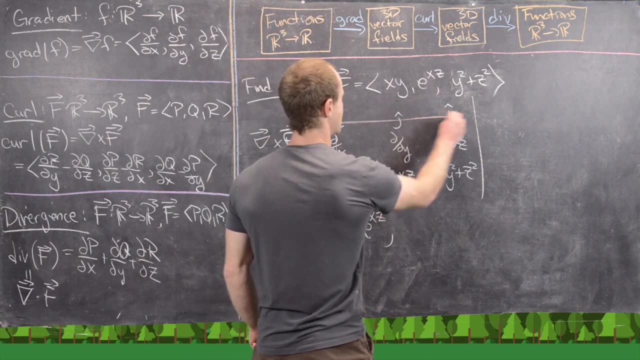 So that's going to be 2y minus the partial with respect to z of this guy. So that's going to be xe to the xz. Now for the second component. we'll cross again the first row and the second column and then we'll do the partial with respect to x of this, which is 0,. 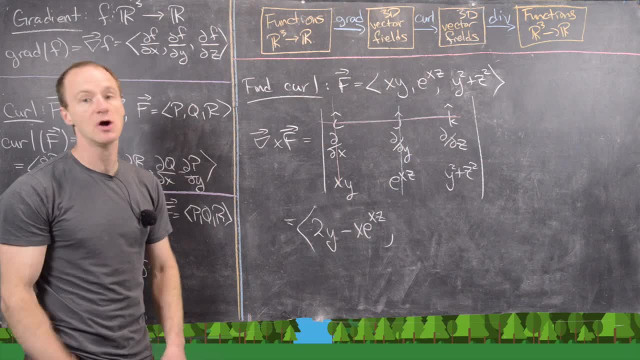 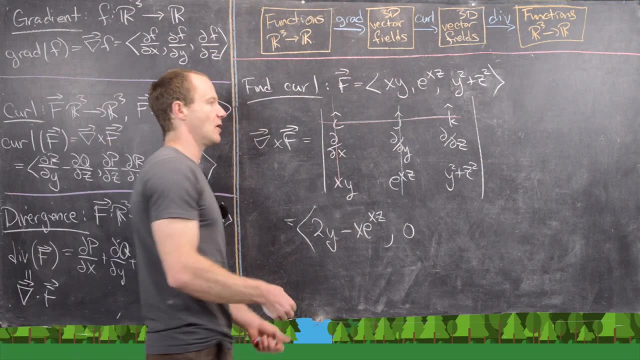 minus the partial with respect to z of this, which is also 0. We would have to flip the sign as well, built into the cross product formula. but either way, you're going to get 0 here. Okay, now last one. 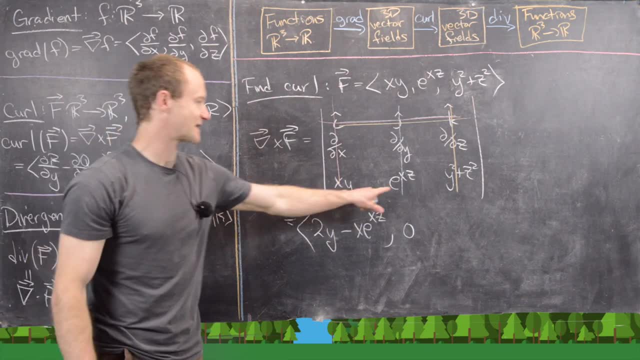 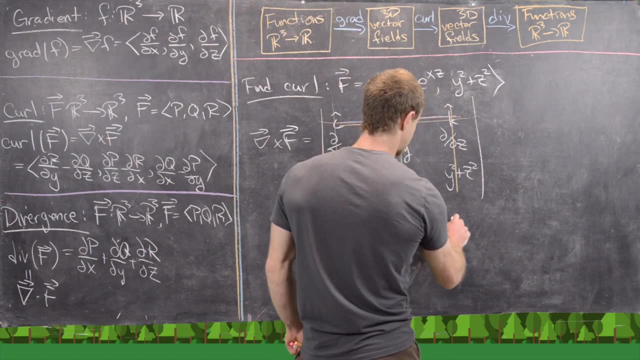 So we'll cross the last column in the first row, Partial with respect to x of this thing. So that's going to be e, sorry z, e to the xz, And then the partial with respect to y of that thing. 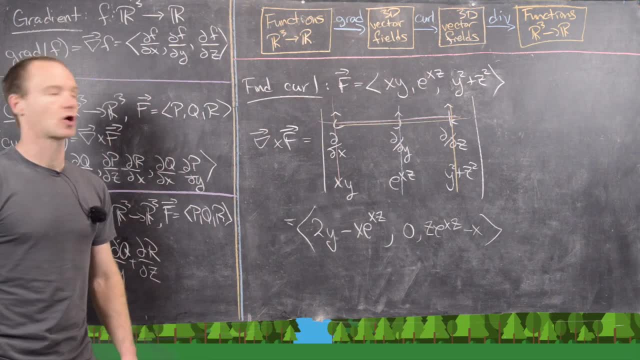 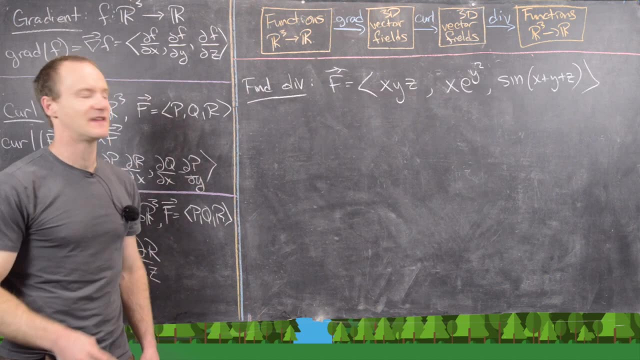 So that's going to be minus x. So that is our curl for this vector field. Okay, so I'll clean up the board and then we'll find the divergence of something. So let's go ahead and find the divergence of this. So we'll use this property that it's del dot f. 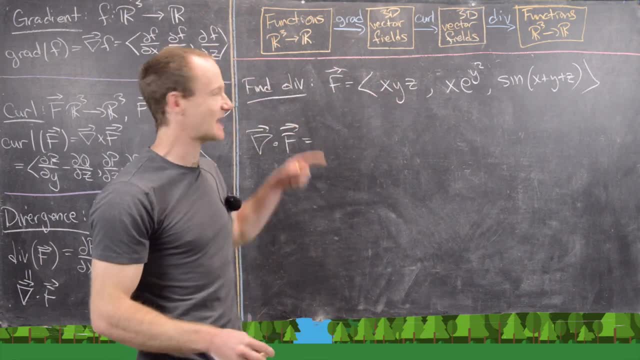 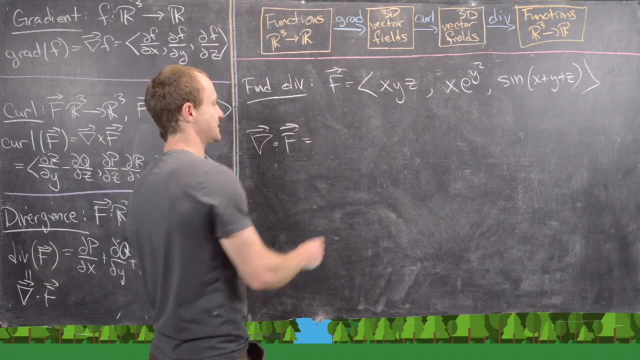 So we need to take the partial of this guy with respect to x, add it to the partial of this one with respect to y, add it with this partial of that one with respect to z. So the partial of this with respect to x. 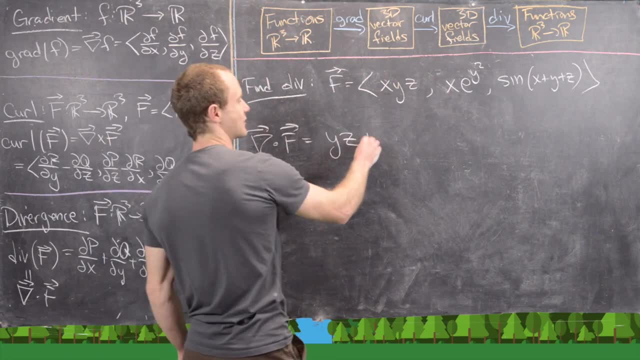 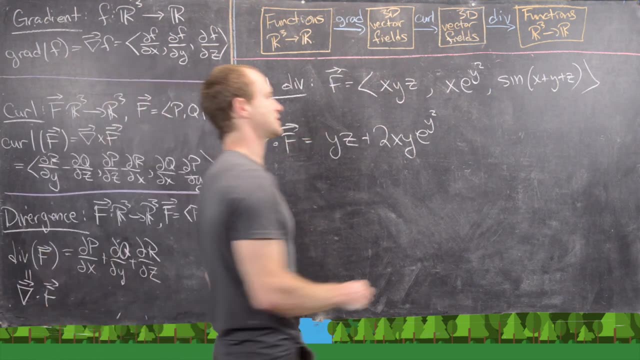 x is yz plus the partial of that with respect to y is 2xy e to the y squared Notice, I had to use the chain rule there, and then the partial of the last one with respect to z is cos x plus y plus z. 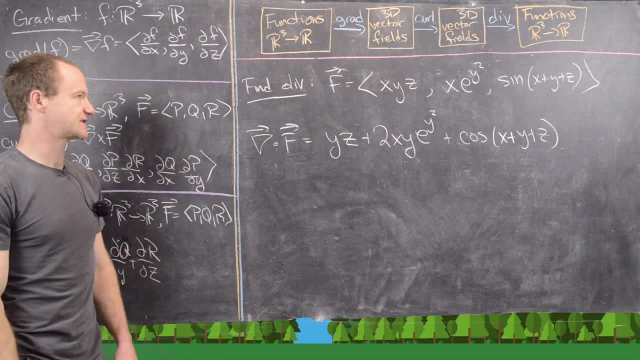 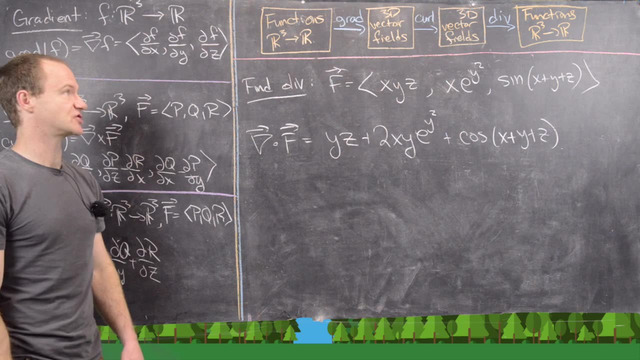 and that's all that we have for the divergence of this vector field. Okay, I'll clean up the board and then we'll talk about some properties of gradient divergence and curl. Okay, so the first result that we're going to look at is about the classification of conservative vector fields. So 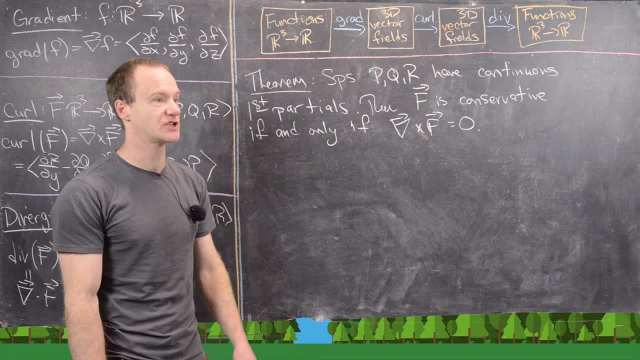 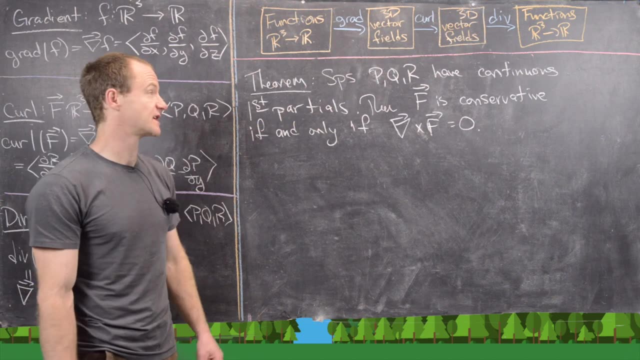 I've got a whole video on conservative vector fields that you can check out what their definition is, although we'll use the definition in this. So what it says is that if p, q and r have continuous first partials, then the vector field f- which I should say this- is made up with component functions. 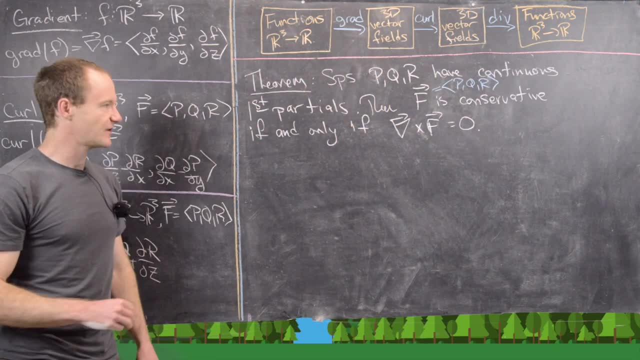 p, q and r is conservative if, and only if, the curl of f equals zero. So let's go ahead and look at the proof of that. So let's go ahead and look at the proof of that. So let's go ahead and look. 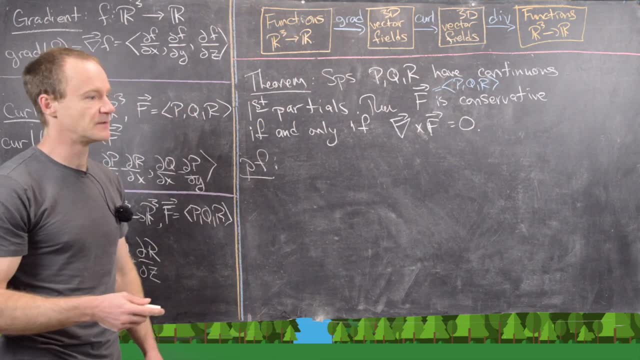 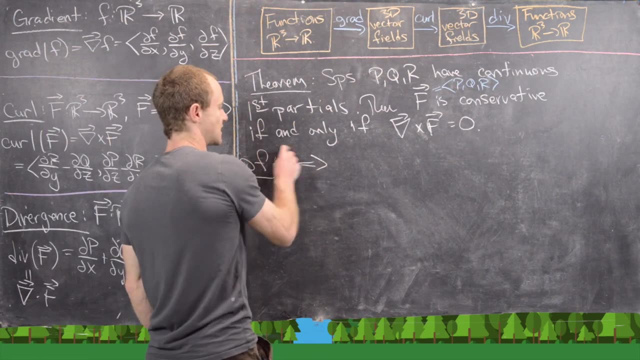 at the proof of one direction of this, We won't do the proof of the other direction, although I will point you towards a hint of how it would work. Okay, so let's go ahead and do this forward direction. In other words, we want to suppose that f is conservative, which is the same thing. 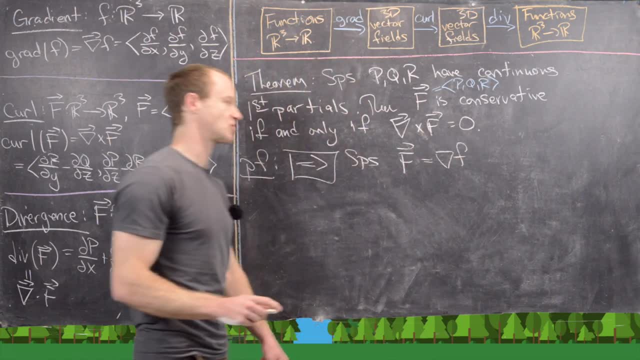 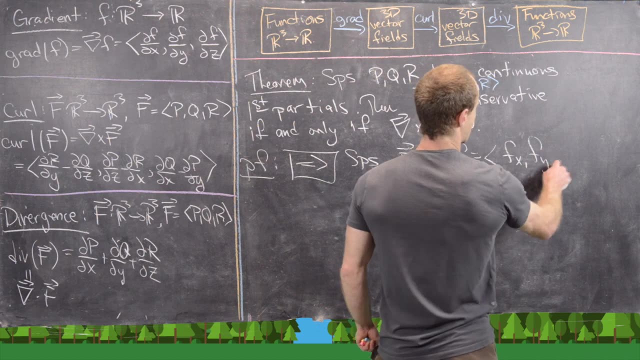 as saying that f equals the gradient of a function, little f. That's the definition of f. being conservative, That means that is equal to f sub x, f sub y, f sub z. It's the so-called gradient of a function, little f. So let's go ahead and do this forward direction. In other words, we 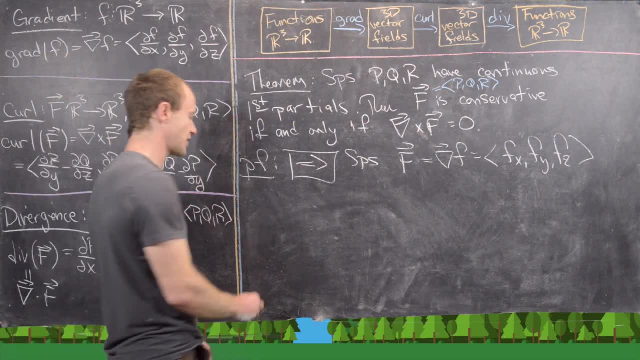 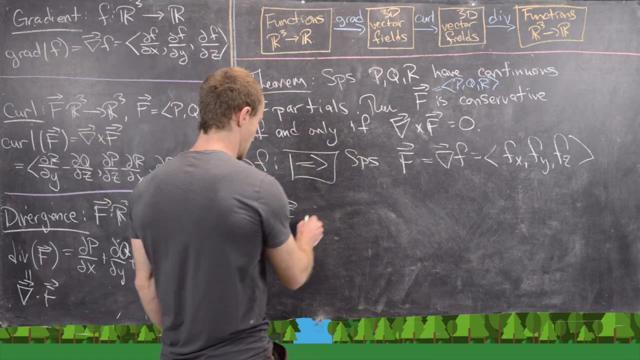 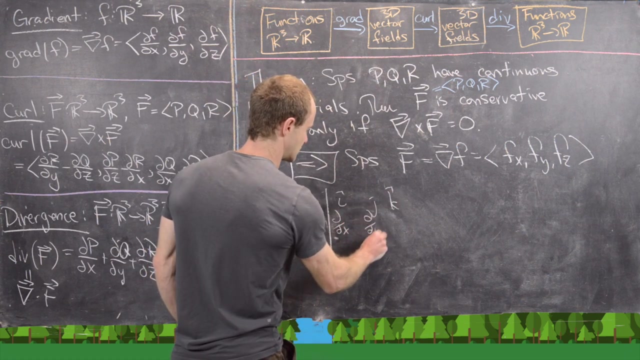 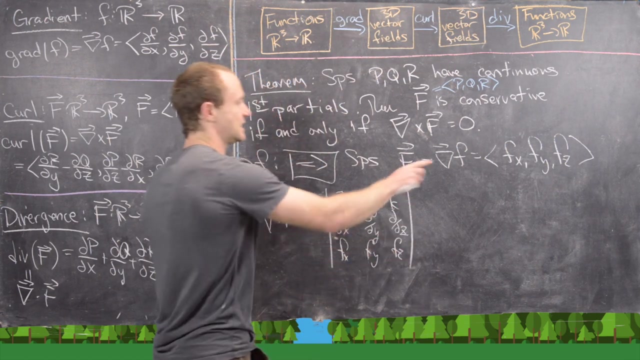 gradient vector field. Now let's go ahead and calculate the curl of f and see what we get. So that's going to give us the determinant i, j, k, and then we have these partials- Partial x, partial y and partial z, And then f sub x, f sub y, f sub z, given that this thing is a gradient vector. 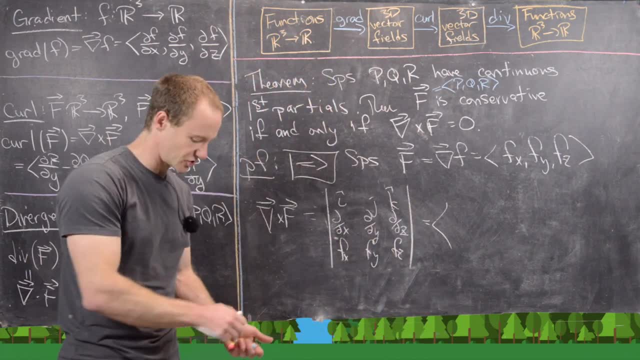 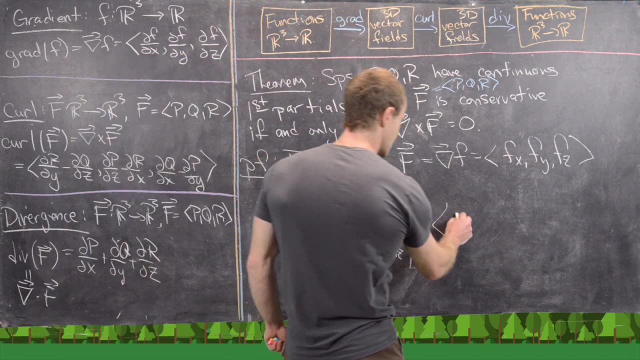 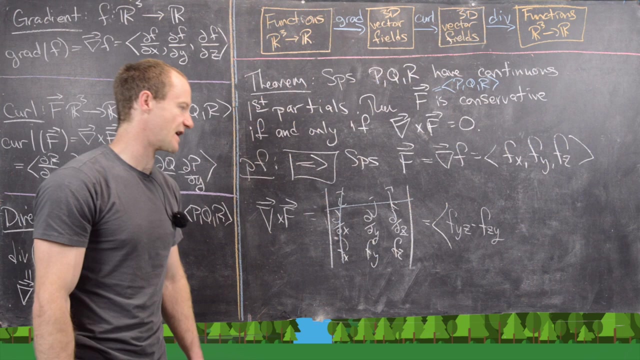 field. Okay, good. So now let's look at the proof of that. So let's go ahead and do this forward direction, The first entry. So, again, just like our example, the first entry will be gotten by doing that cross. So that is going to be f y z minus f z y by. this is the partial with respect to y of that, The. 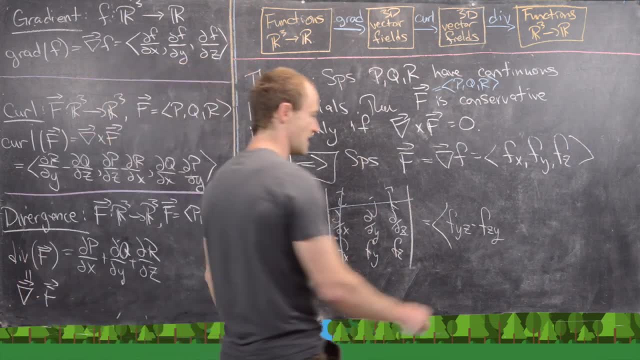 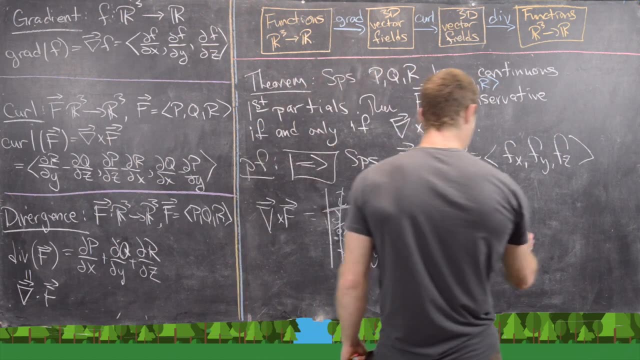 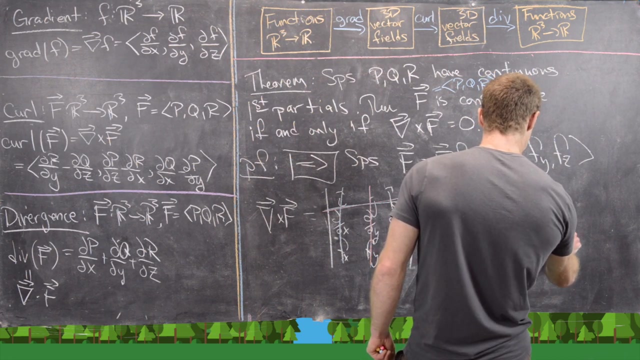 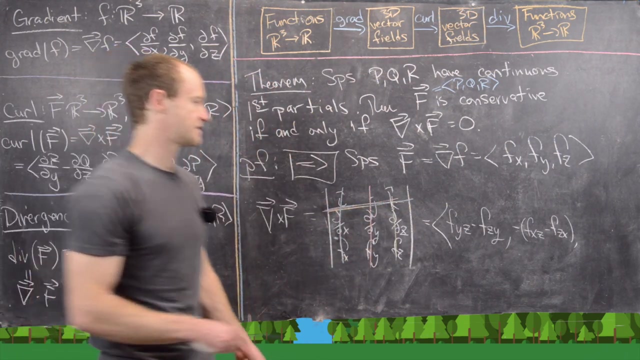 partial with respect to z of f sub y. And then let's see what our second one is. So that's going to be the second column in the first row, So that'll be negative, the f sub x z minus f sub z x. So, and then finally the last column in the first row, So that'll be f x y. 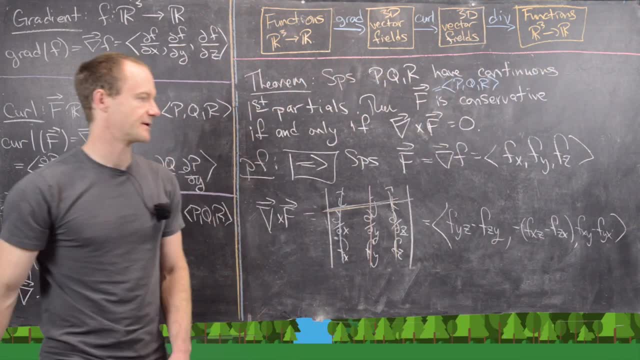 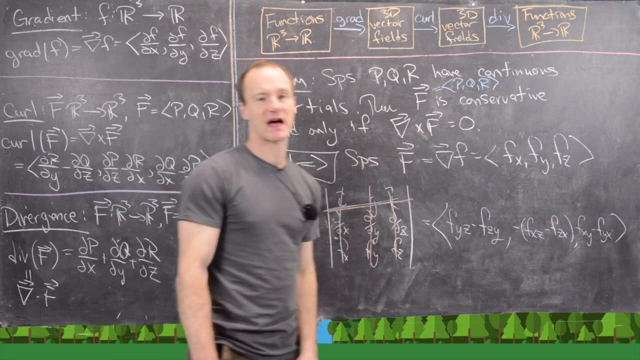 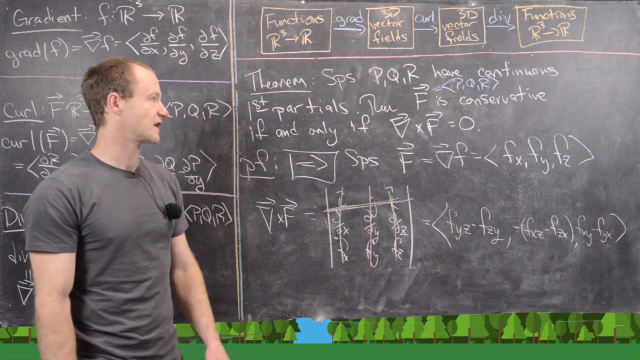 minus f, y, x. Okay, good, But now since p, q and r have continuous first partials, that means f has continuous second partials, Because the second partials of f are the first partials of p, q and r, Which means that the order of differentiation doesn't matter by 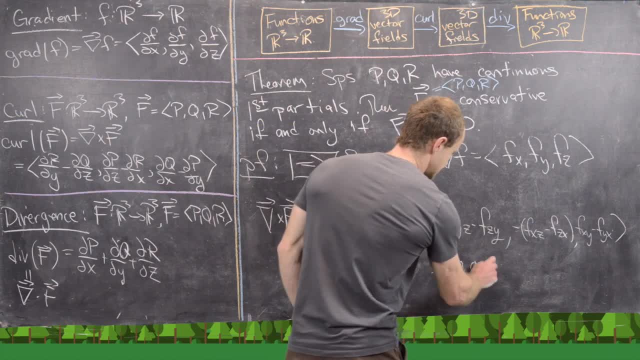 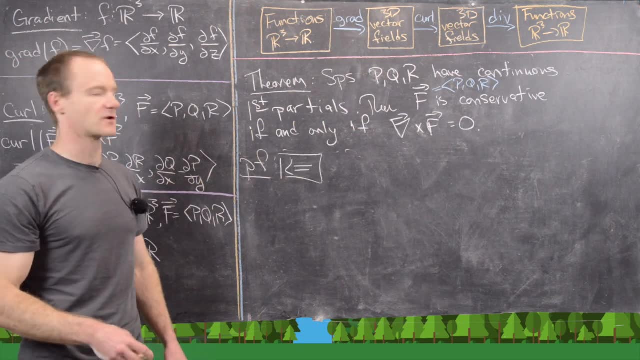 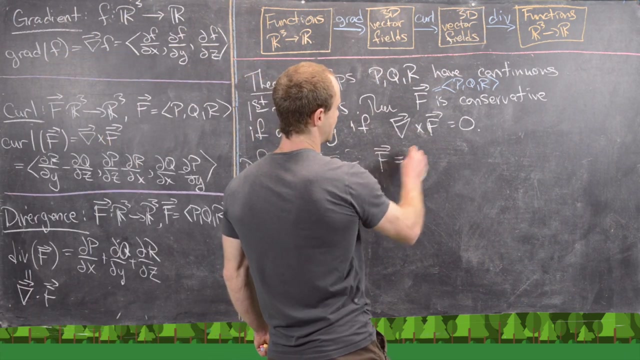 Clairaut's theorem, Which tells you that this is exactly the zero vector field, Which is exactly what we need for this direction. So now let's look at the reverse direction. Like I said, we're going to restrict it to the plane. So let's suppose f is a two-dimensional vector field. 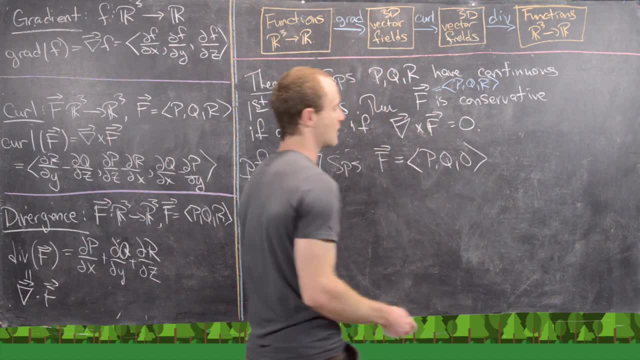 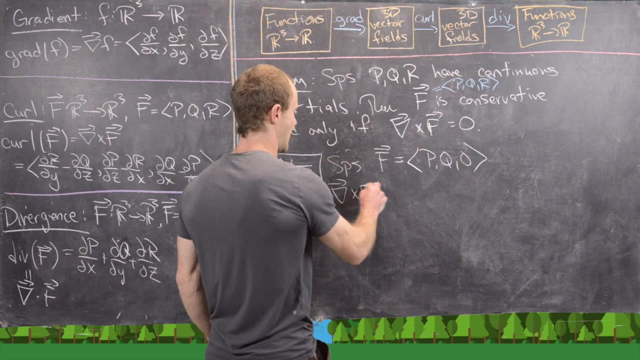 That means we're going to write it as p, q comma zero, And p and q only depend on x and y, And so that means we can take the curl of f, which we've decided is equal to zero, given the fact that we're assuming that. So that is. 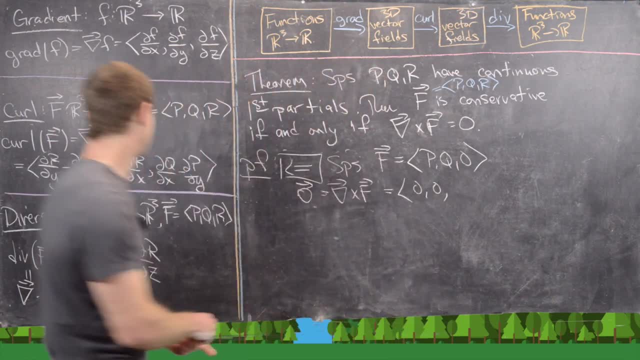 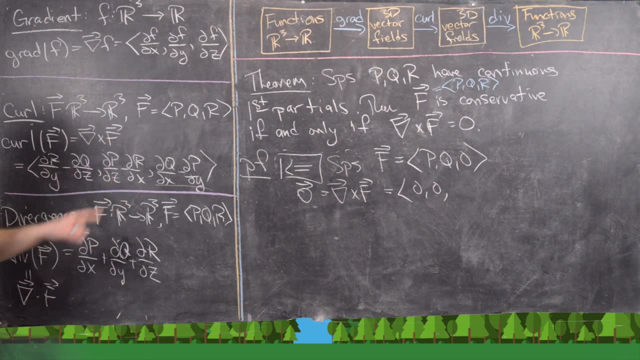 going to be equal to zero comma. zero comma- this guy right here- Because all we have are the component functions p and q, And then p doesn't depend on z and q doesn't depend on z, So we don't get anything for those first two components. 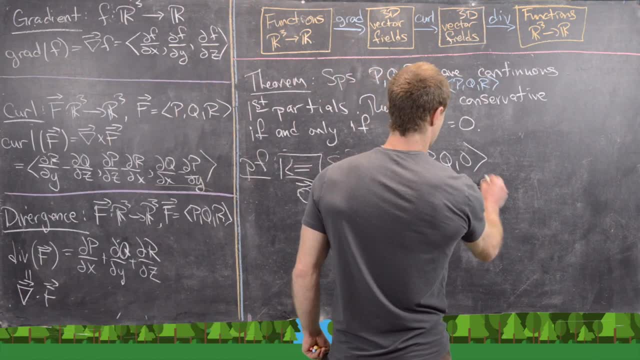 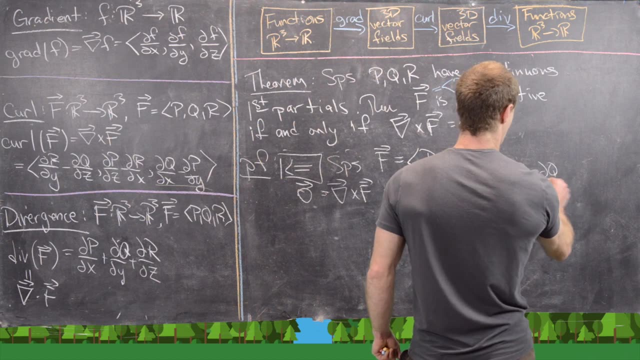 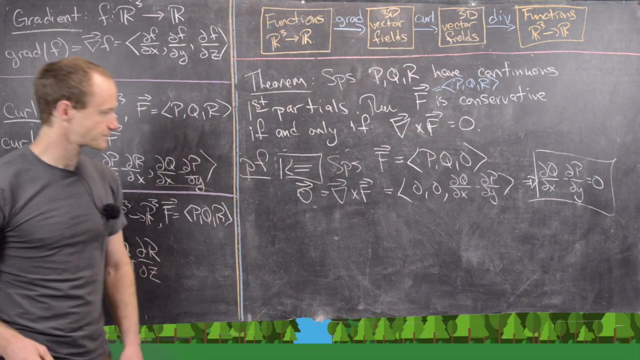 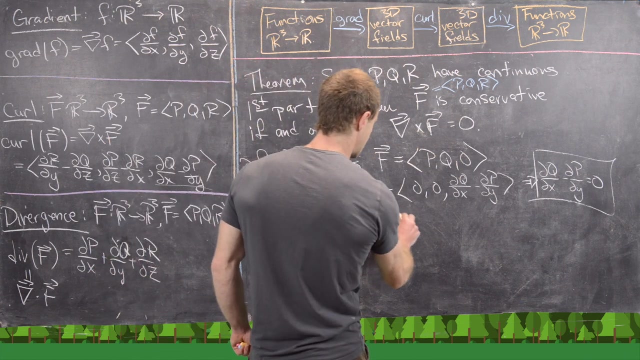 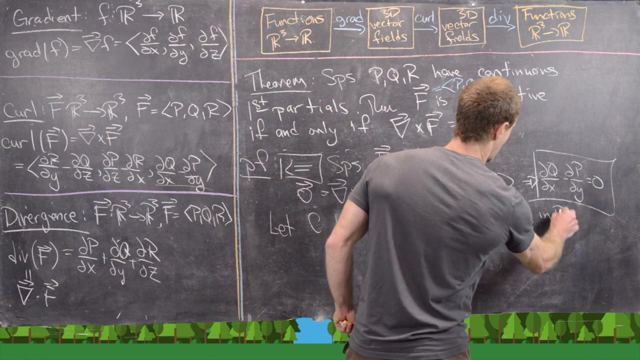 So we just have partial q, partial x minus partial p, partial y. So in other words, we know that partial q, partial x minus partial p, partial y equals zero. Great, So now the next thing that we want to do is let c be a simple closed curve in the plane. 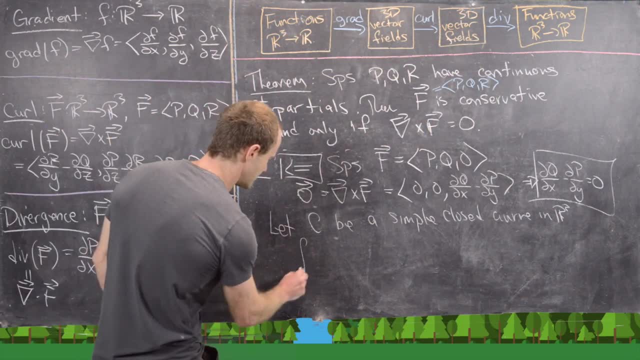 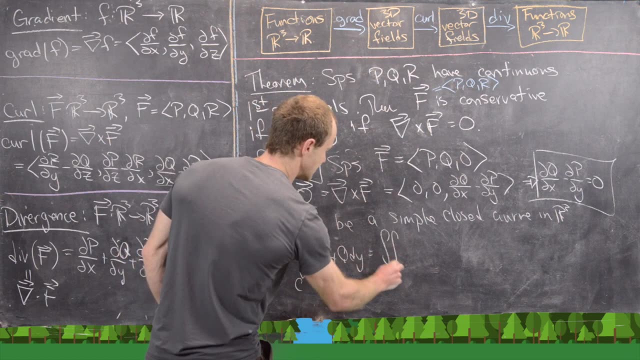 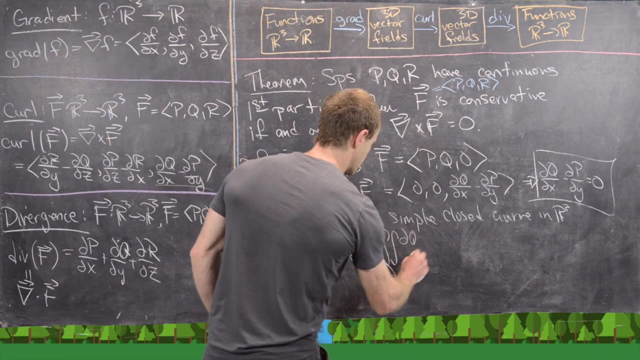 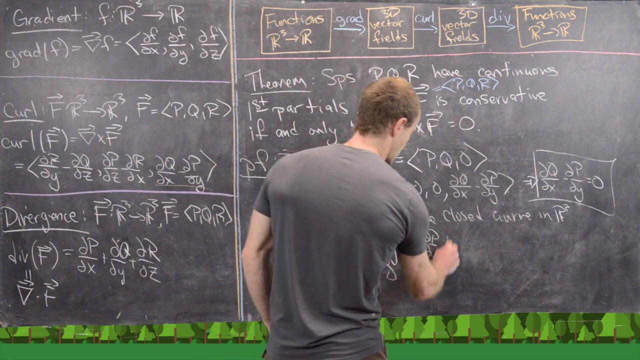 Great. And then notice that the integral over c of pdx plus qdy is going to be equal to the double integral over d, where d is the region being bound by c of dqdx minus dpdy. And here we have that this is equal to zero. But when you 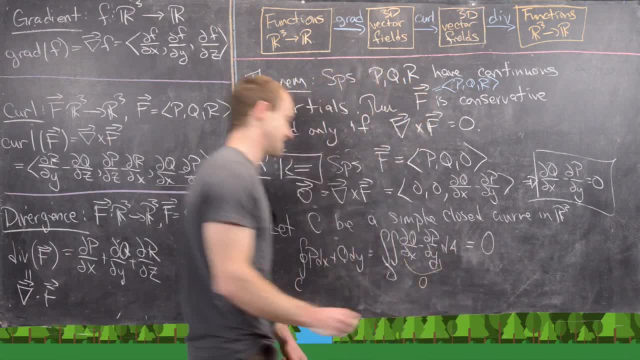 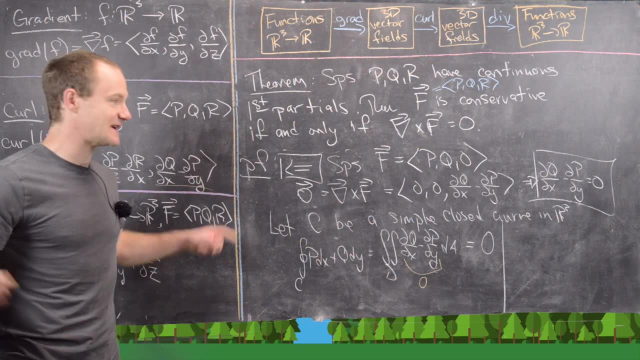 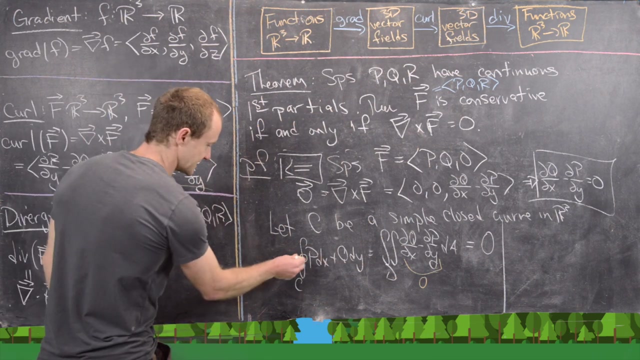 integrate zero over anything, you're going to get zero. So this is equal to zero. So what that tells us is that, since c was chosen to be any simple closed curve, we know that integrating this vector field, which notice this, is the same. 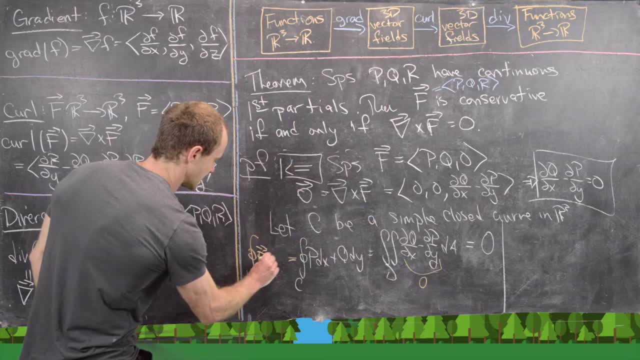 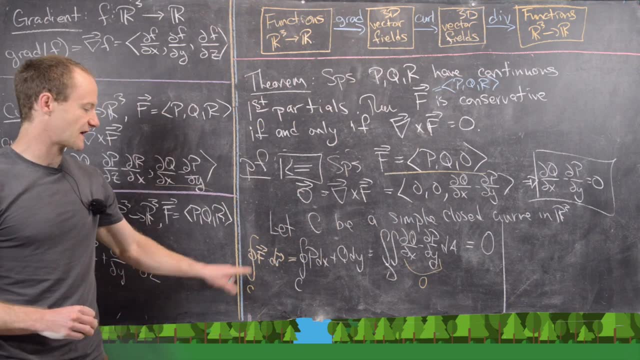 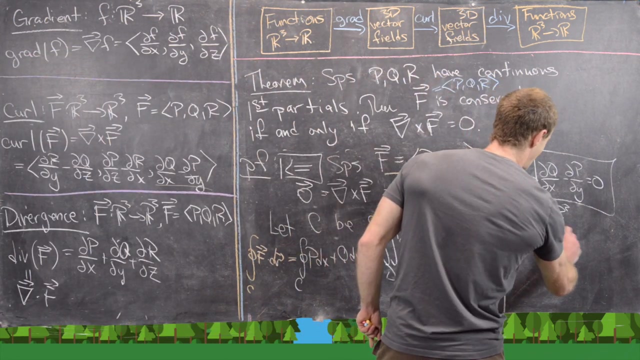 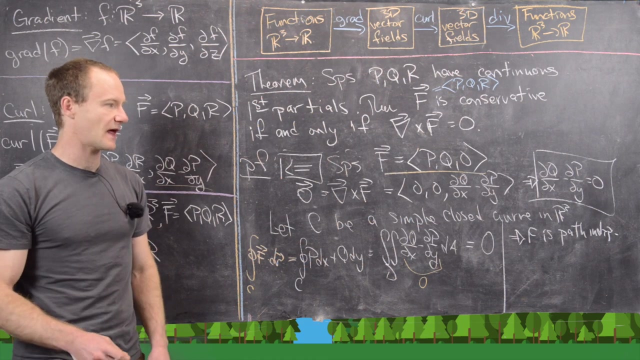 thing as integrating the vector field f dot dr. given that f is defined by this pq0, integrating this vector field over any simple closed curve and getting zero is the same thing as saying that F is path-independent. But I've got another video where I prove that in the plane. 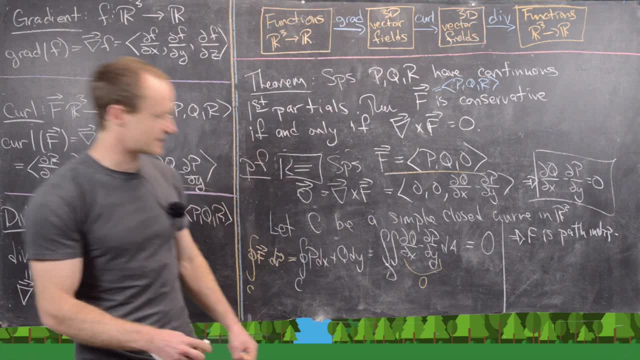 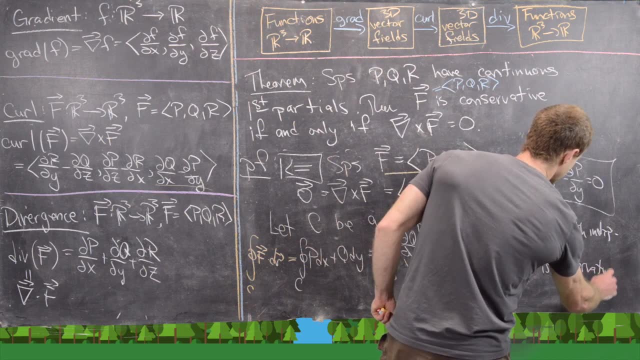 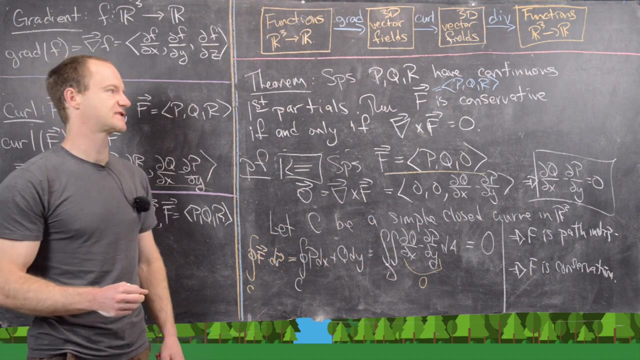 path-independence is equivalent to being conservative, So that means that F is conservative. So notice, I've only done this in the plane and I've really waved my hands at it, but this is kind of the idea for how this direction goes. 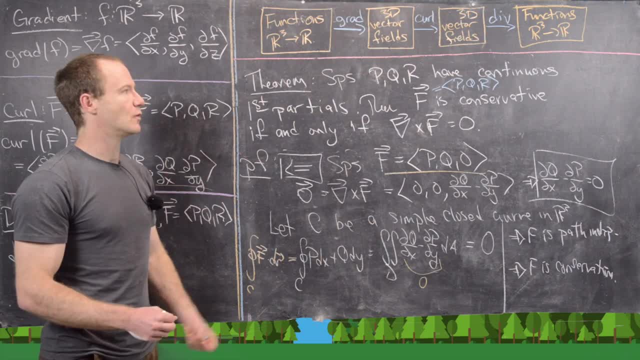 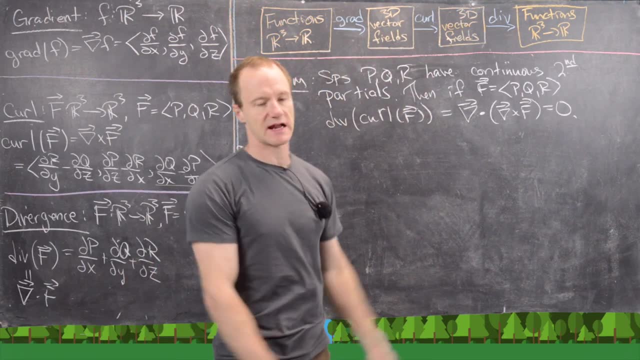 Okay, so I'm going to go ahead and clean up the board, and then we'll look at one more property. Although we didn't phrase it like this, we just looked at how the gradient and the curl interacted with each other, and we'll summarize that in a bit. 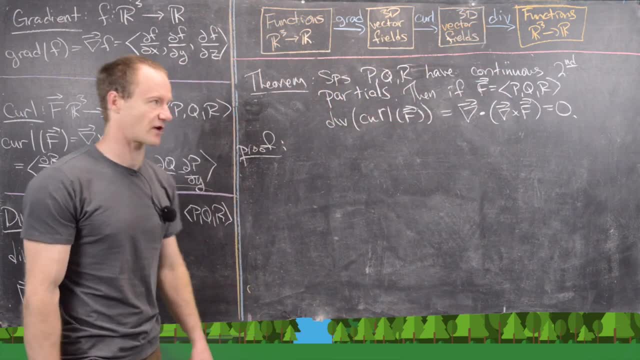 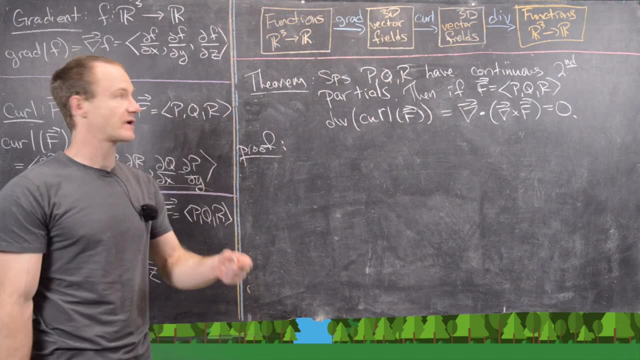 So now we want to look at how the curl and the divergence interact with each other, and they interact in the way described by this theorem. So let's suppose that P, Q and R are three variable functions that have continuous second partial derivatives. 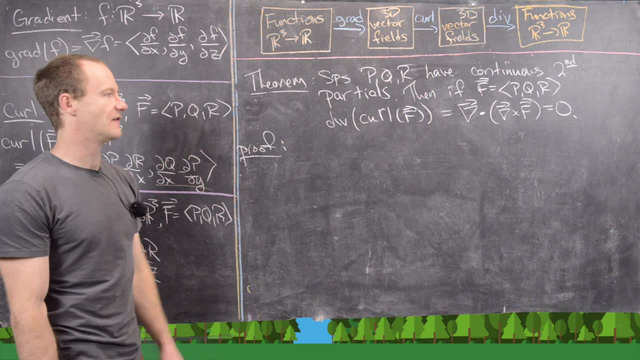 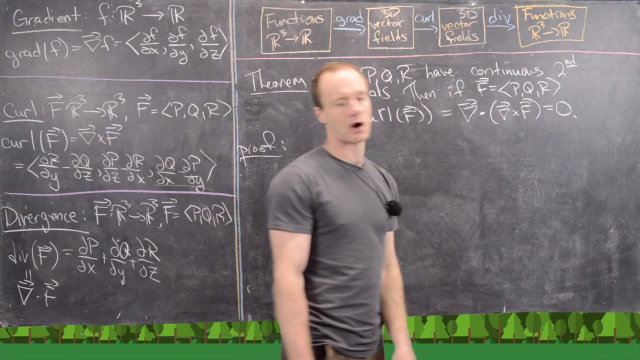 Then if we make a vector field out of them and we'll call it F, the divergence of the curl of F equals zero. In other words, del dot del cross, F equals zero. Okay, so let's see how this proof goes. 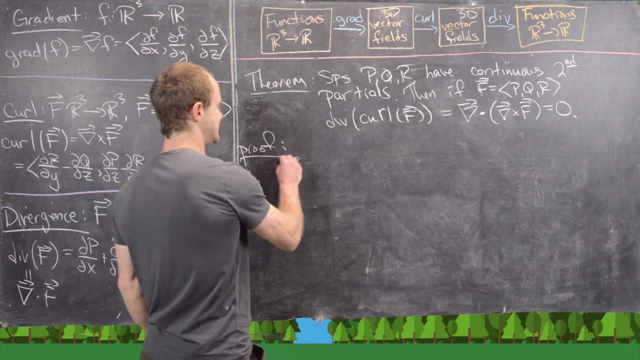 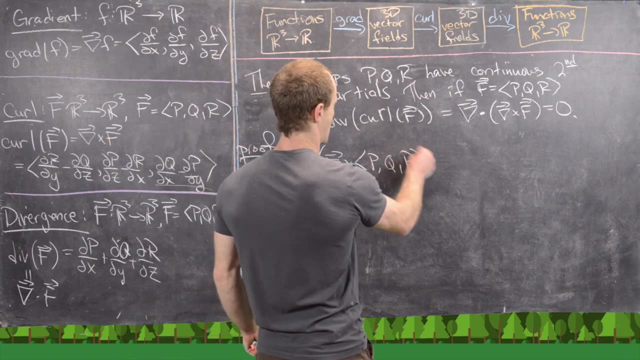 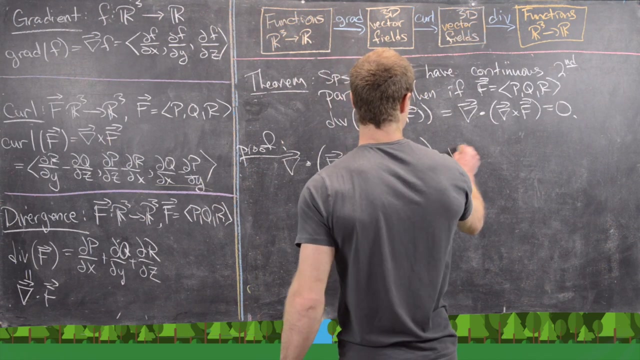 So we need to find del dot, del cross, P, Q, R, Like that. Okay, so instead of writing this all out, I'll just take this definition. so we need to do del dot, this vector field, over here, because that is how the curl is defined. 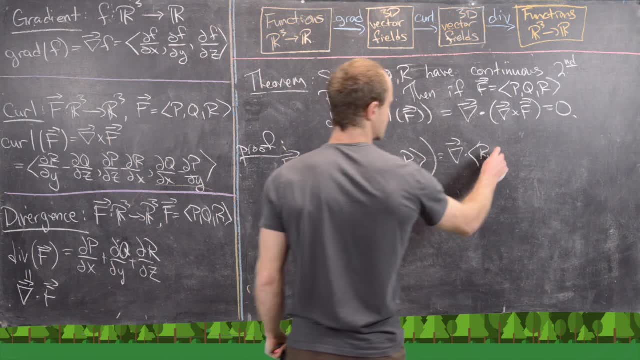 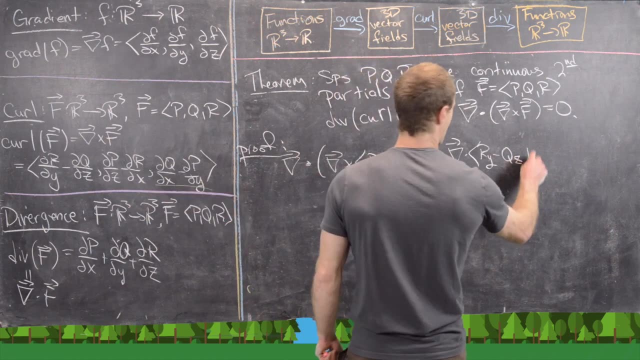 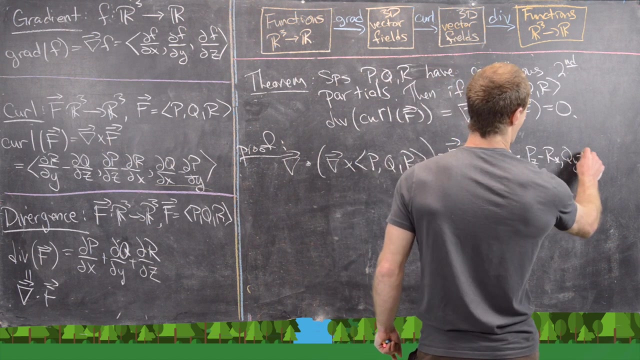 So I'm going to use the subscript notation for partial derivatives just to make it shorter. So we have R Y minus Q Z, And now, next, we're going to have P Z minus R X, And then finally, we're going to have Q X minus P Y. 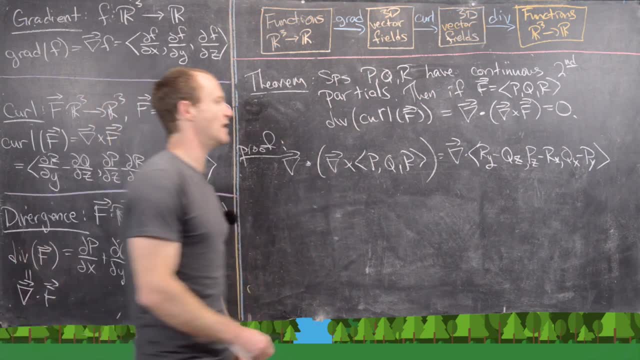 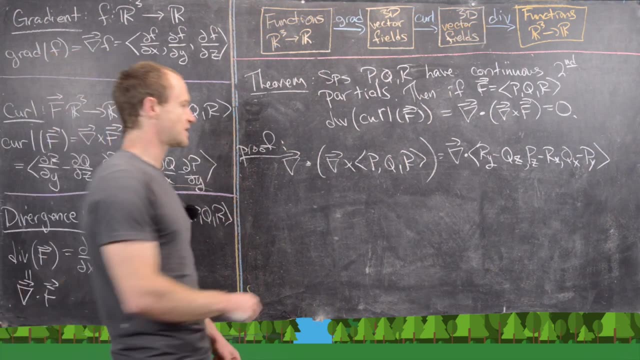 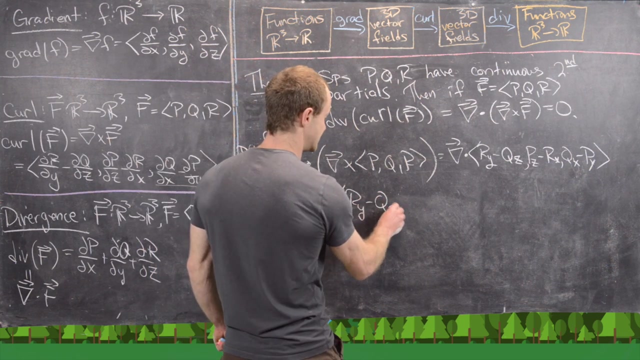 Okay, so that would be the curl of F. Now the next thing we need to do is take the divergence of that. So in other words, we need to take the partial, with respect to X, of that first component, which is R Y minus Q Z. 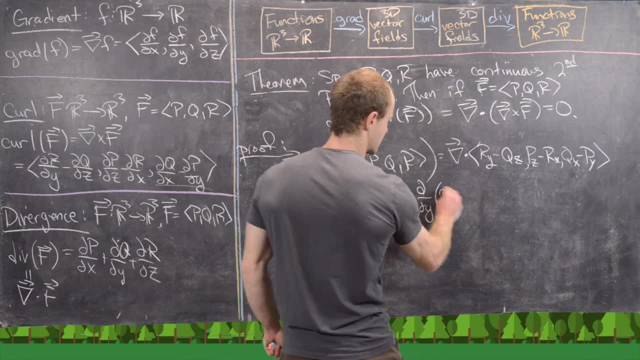 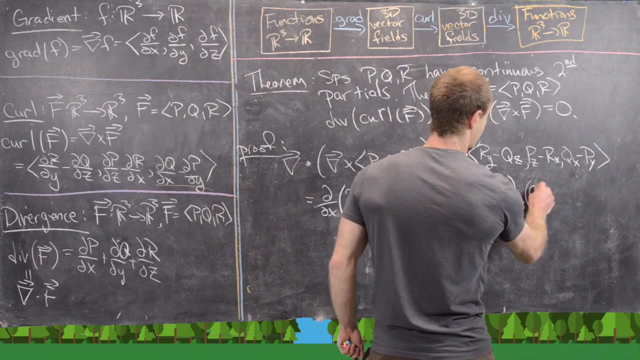 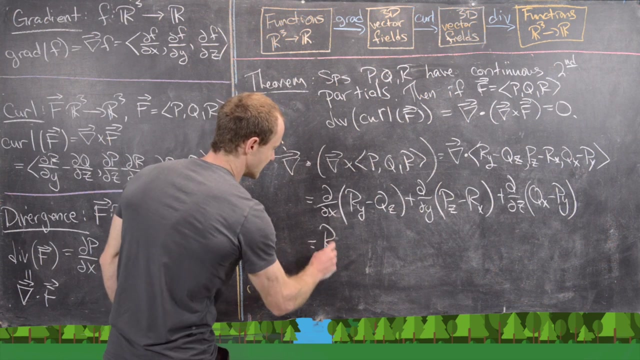 plus the partial, with respect to Y, of that second component, which is P Z minus R X, And then, finally, the partial with respect to Z, of that third component, which is Q X minus P Y. Okay, fantastic. So notice, that's going to give us R X Y minus Q X Z. 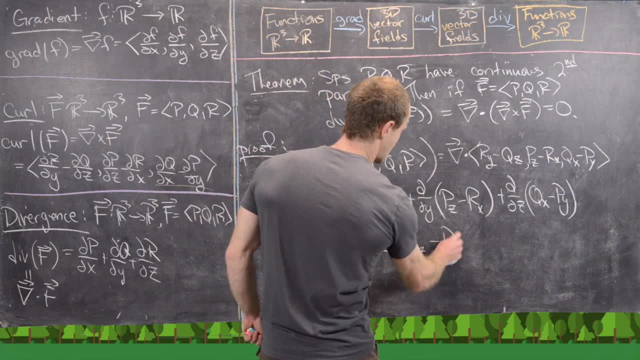 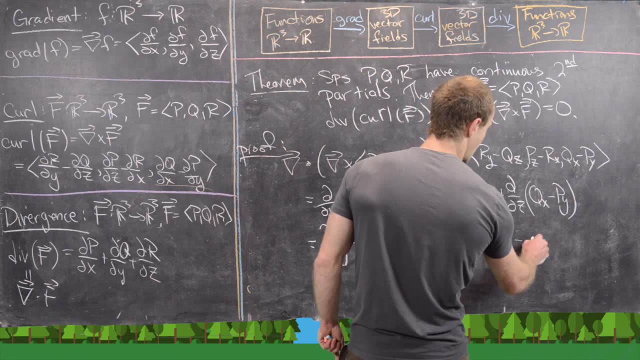 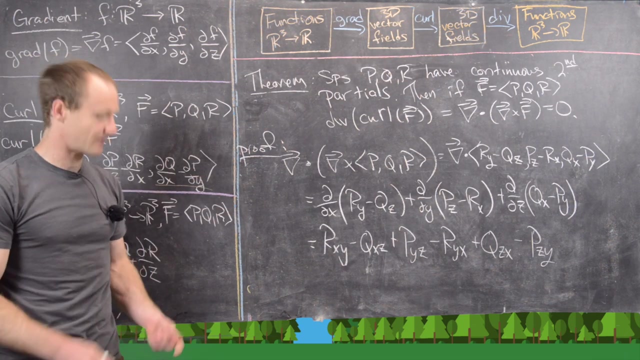 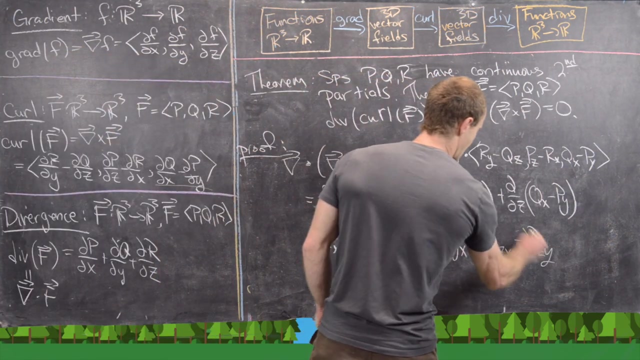 plus P Y Z minus R Y X, and then plus Q Z X minus P Z Y. But then by Clairaut's theorem, since we have second continuous partial derivatives, we can change the order of derivatives and that's going to give us: that guy cancels that guy. 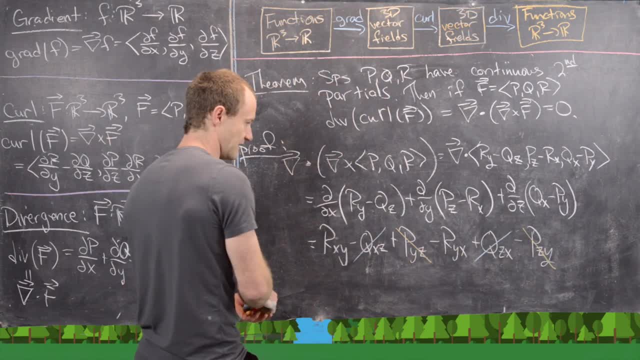 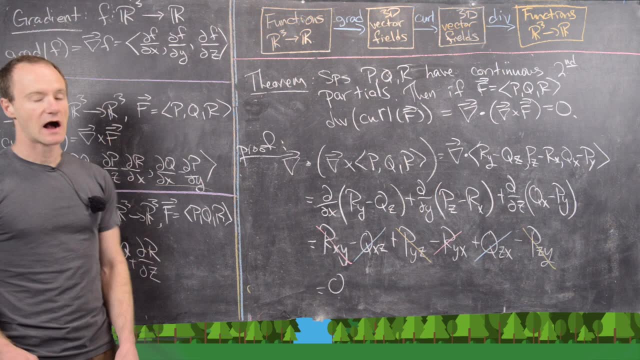 this one is canceled by this one, and then, finally, this one is canceled with this one, and then we get zero. Okay, good, So I'll clean up the board and then provide a summary of how these things interact with each other. So let's summarize what we've just seen.